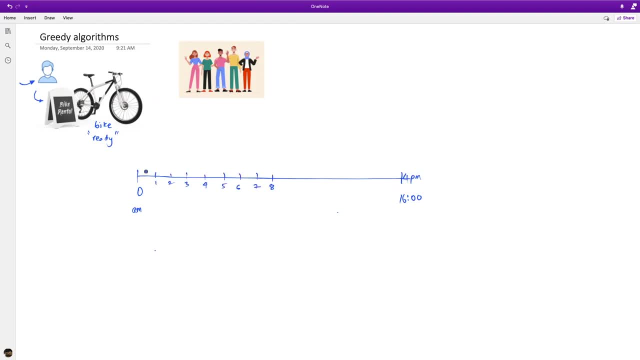 until the 4 pm. so let me number these hours. So we have total 17 hours slots: first slot, second slot, third slot and so on. Say there are 11 people wanting to rent the bike wanting to rent the bike for the next day. that is beginning from midnight until 4 pm. 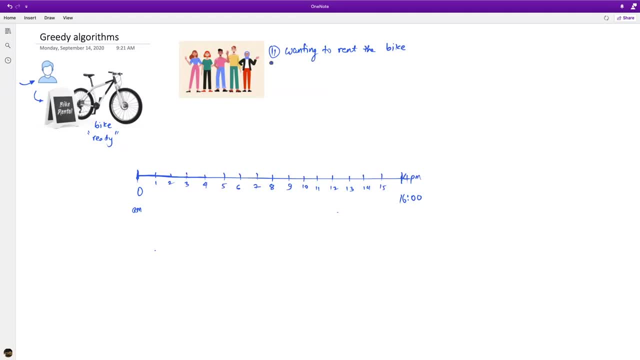 Let's see what are the demands of these 11 people, That is, during what duration they want the bike to be rented further. The first person is wants the bike to be rented from 1 am to 4 am. from 1 am to 4 am. this is. 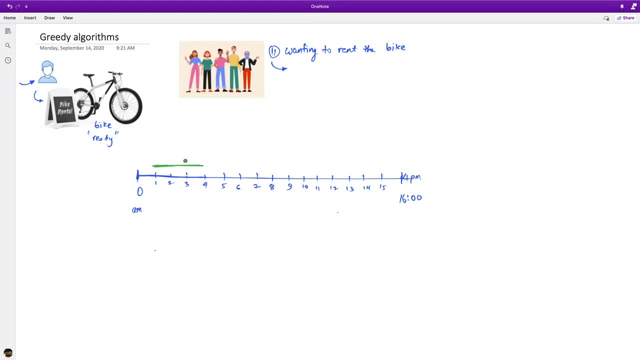 the first demand. the second person wants the bike from 3 am till 5 am. third person wants the bike from midnight until 6 am. fourth person wants the bike from 5 am to 7 am. another person wants the bike from 3 am to 9 am. 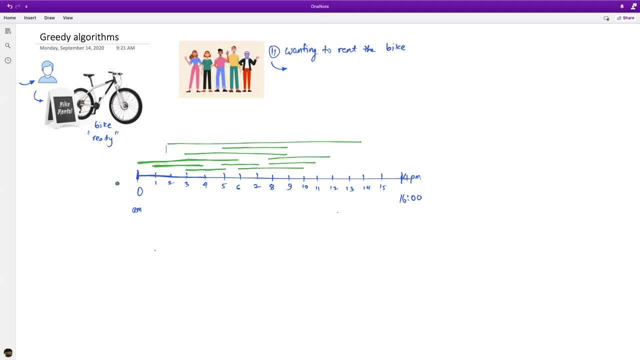 and the last person wants the bike from noon till 4 pm. now, since you own the bike rental company, what you would like to do is rent this bike to the maximum number of customers. that is, your goal is to rent the bike to maximum number of. 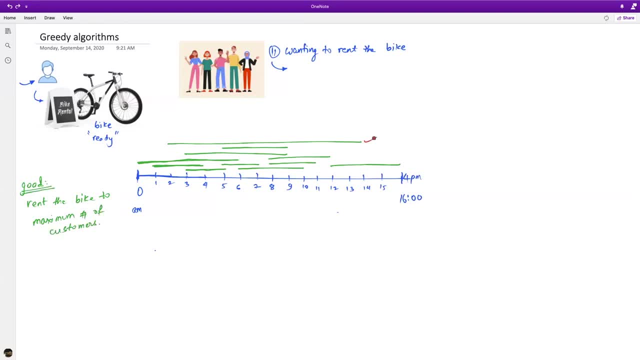 customers. now, obviously, if you rent the bike to this guy, you will not be able to rent the bike to almost any other person, right? so your goal is not met. you might choose to rent the bike to this person and then, after that, you could rent it to this guy and then to this guy, eventually serving three. 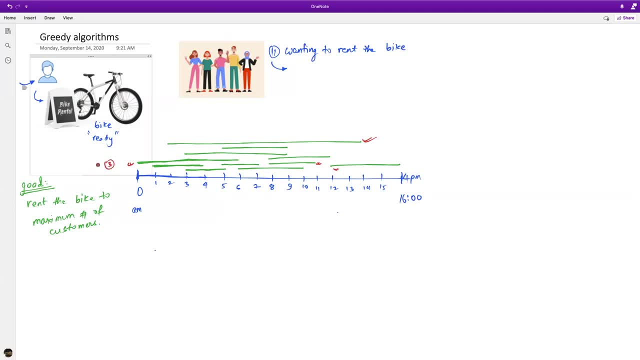 customers, so that probably is also not the best choice. so, in this way, what we would like to do is find a way or come up with an algorithm that allows us to find what is the maximum number of customers that I can serve you, given this schedule of demands and the total time slot that i have my bike available formally. 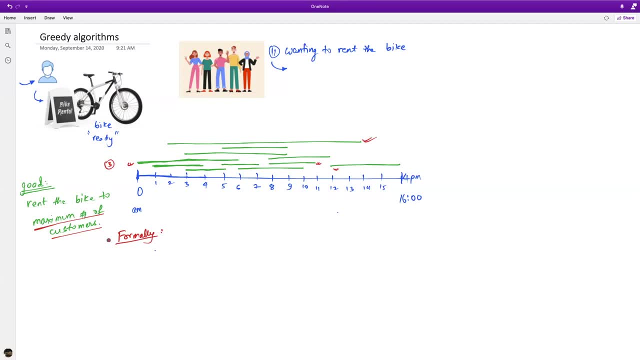 we say that in the activity selection problem we have a set of proposed activities. in this case we have 11 activities which we represent by using this capital letter: s equals. all the activities are represented using this letter: a1, a2, a3, up to a n. in this case, we have 11 activities. 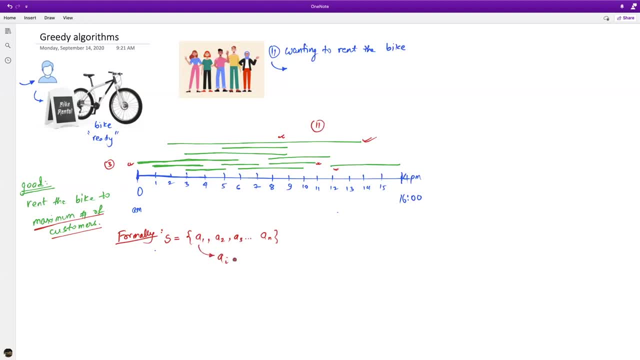 here now. each of this activity ai. activity ai has its own start time s? i and its own finish time f? i. so obviously always s? i will be smaller than finish time fi. we say that two activities, a and AJ, are compatible if the intervals for AI and AJ do not overlap. so AI may. 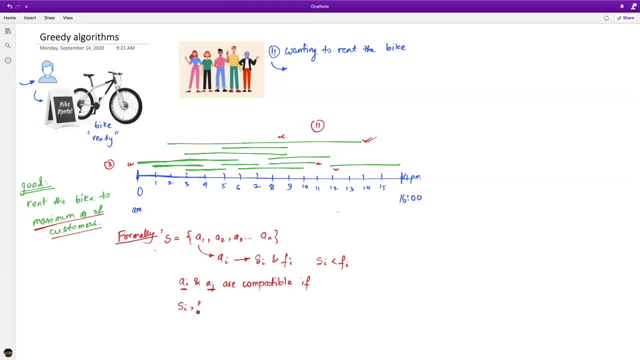 have an interval such as this goes from SI to FI and AJ may have an interval, for example SJ to FJ. so if these two don't overlap don't overlap, then we say that these two activities are compatible. so here, activities such as this one and this one are compatible, whereas activities such as this one and the 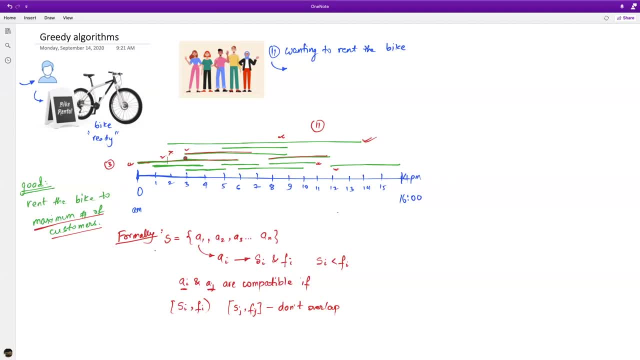 second one. so this and this are not compatible because they overlap. in other words, for two activities to be compatible, we should be such. it should be such that we should be able to share our resource- in this case, bike- to both the activities, and the goal for us is to select a maximum. 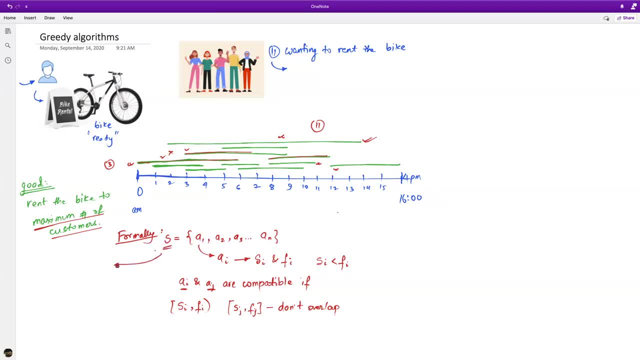 size of activities that are compatible with each other and we should be able to share our resource- in this case, bike to both the activities and the goal for us is to select a maximum size. so, from all of these activities, what we would like to do is select a maximum size subset of mutually. 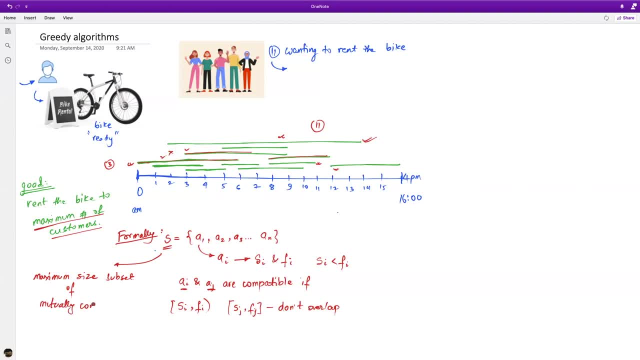 compatible activities, mutually compatible activities. so, in other words, what we want to do is from this set, as we want to obtain a smaller set s in which all the activities are mutually compatible to each other. now I can create a table to put all the activities into a single place, such that they are sorted by their